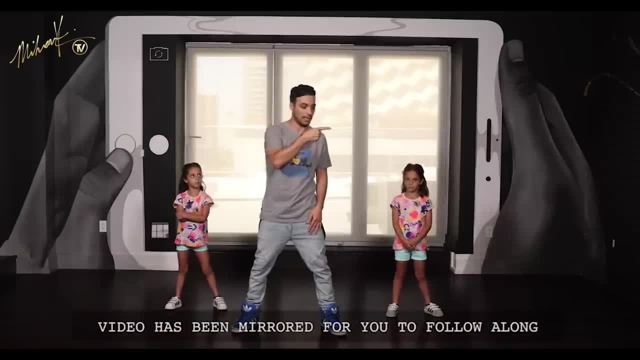 The arms are crossed and then the head goes right, left, and then two times to the right side, And then left right, two times to the left side. Let's do it again, girls, Here we go, Arms crossed, Feet apart, Five, six, seven, eight. 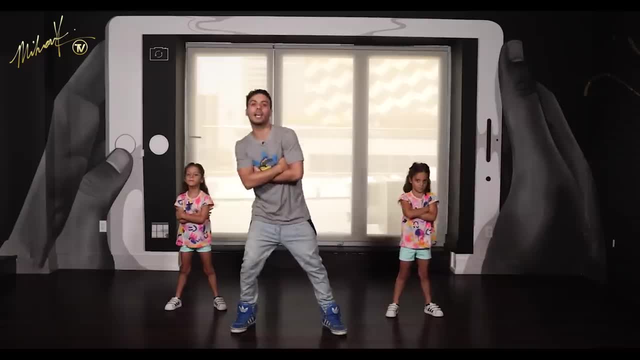 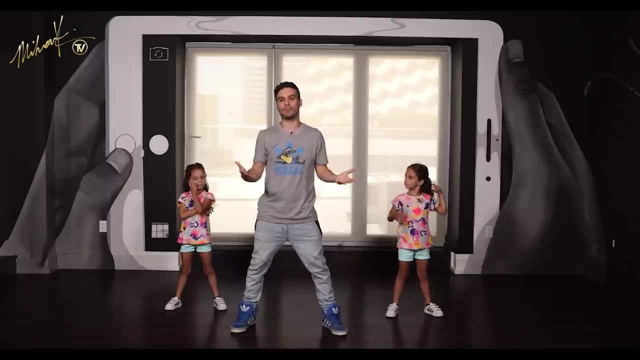 Go right, left, right, Right, left, right, left, left. Good, Let's do it one more time Again. I just put a lot of energy to it. The steps aren't going to be easy. It's just all about the energy and the vibe. 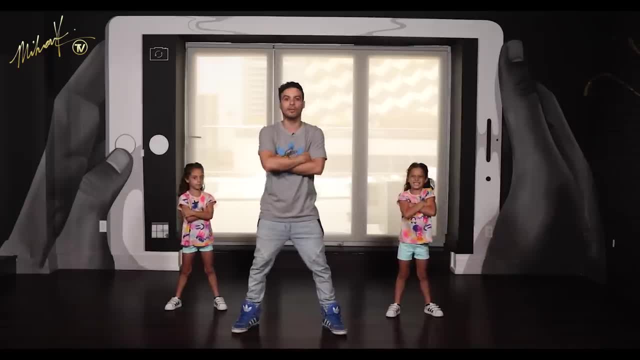 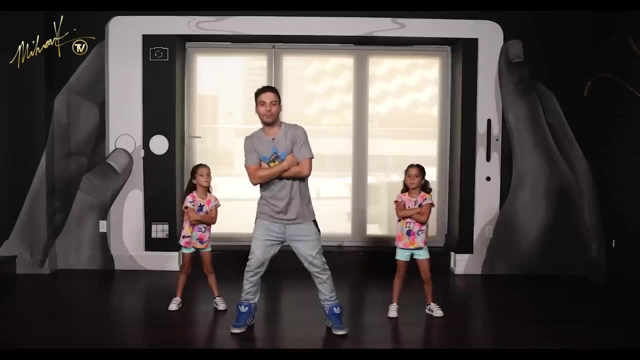 Okay, girls, Let's go a little bit more stronger and a lot more energy. Here we go. Six, seven, eight Go, bounce, bounce double and bounce, bounce double. Good, Let's do it one more time. Here we go. 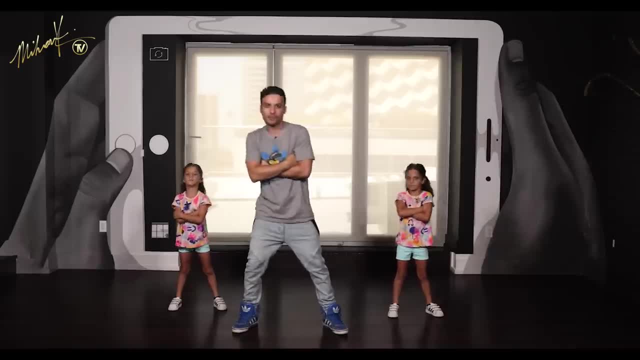 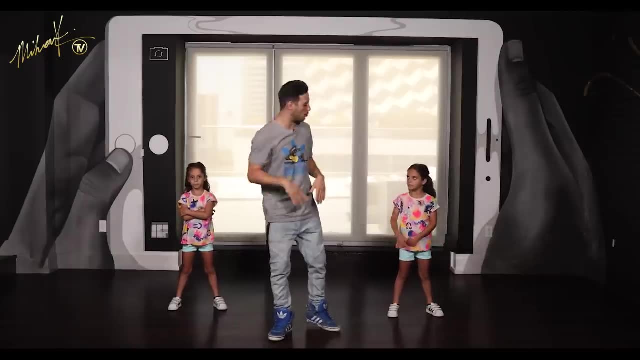 Five, six, seven, eight. Go one, two, three, four. One, two, three, four. Good, So pretty simple step for the first one. Let's do it one more time. I'm going to step back, girls, You stay in the front. 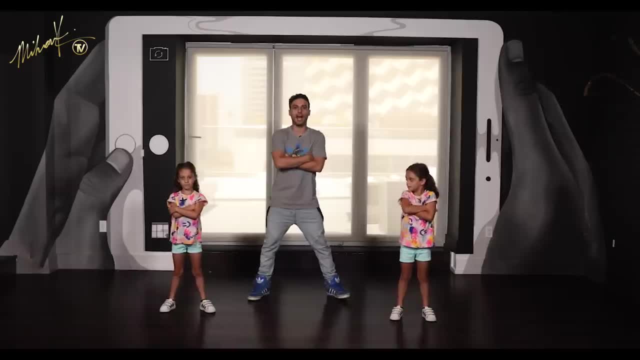 Here we go, Arms crossed, Feet apart. Here we go. Five, six, seven, eight Go right, left, right, right, left, right, left, left, Good. So the important thing here is to move the head on. beat bringing it up, so you're. 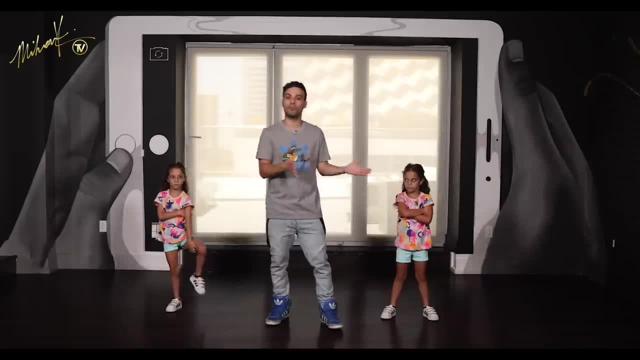 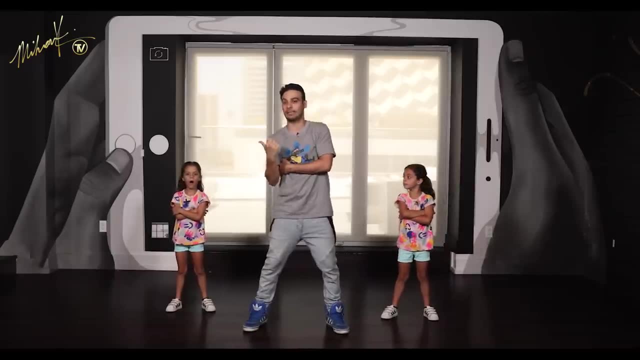 kind of bouncing up on every single count, And also you want to make your lean big. okay, If you can lean more, you can lean more. Some kids might be a little shy and might hold back a little bit. Yeah, like this one here. But at the 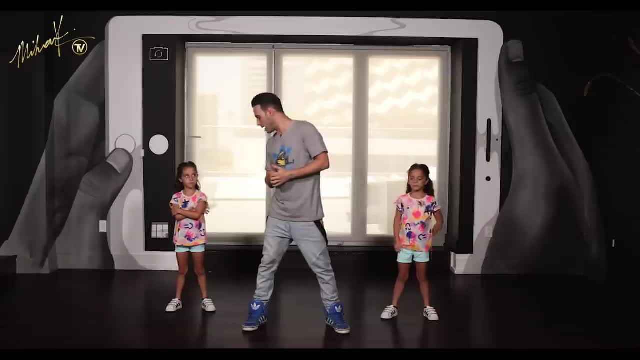 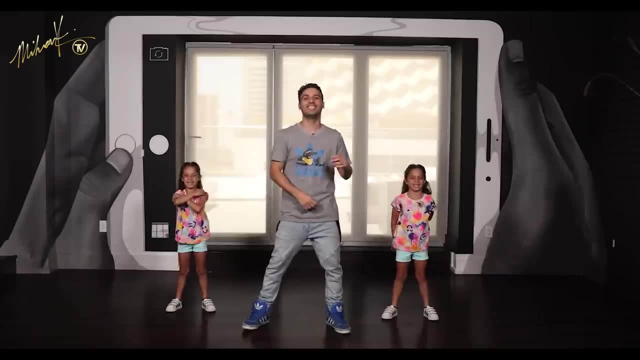 end of the day, it's all about just moving and having fun. Let's do it one more time and then we're going to move on to step number two. You ready, You ready, All right, Here we go. Five, six, seven, eight. 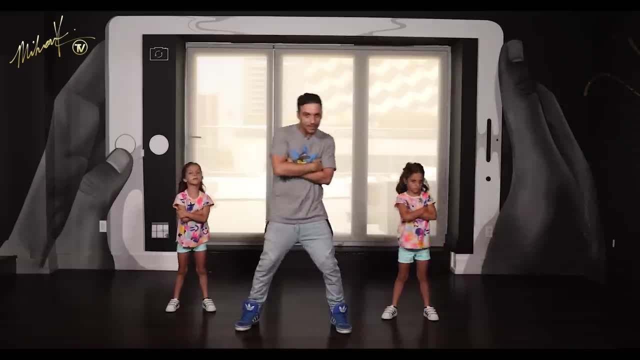 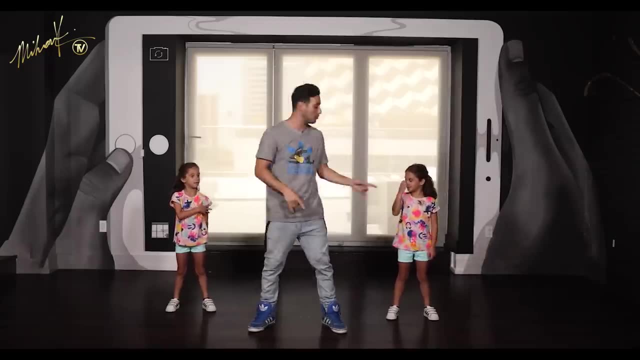 Go one, two, three, four, five, six, seven, eight. Good, Here we go, Moving on to step number two. For step number two, let's start with the arms first. okay, Arms, go out and cross Out, cross out, cross out, cross. Very simple, We're. 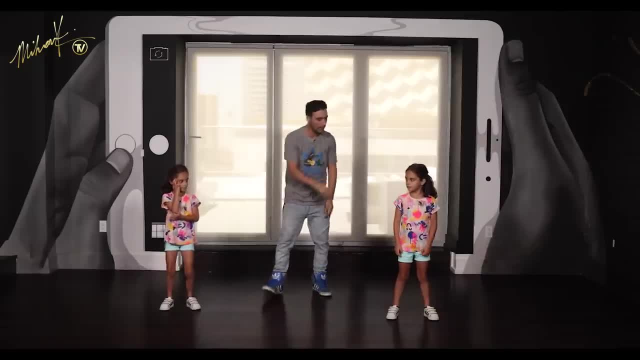 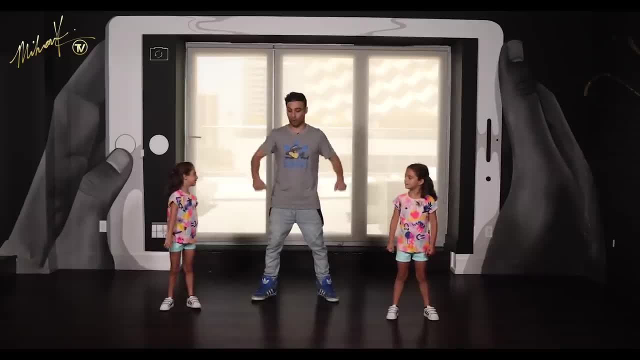 swinging these arms. right now, let's try not to swing and go up down, up out. yeah, not a swing, but up and out, yeah. so let's try it together. here we go. five, six, seven, eight we're going. 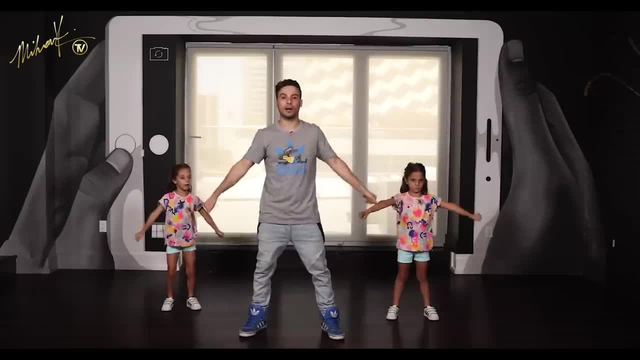 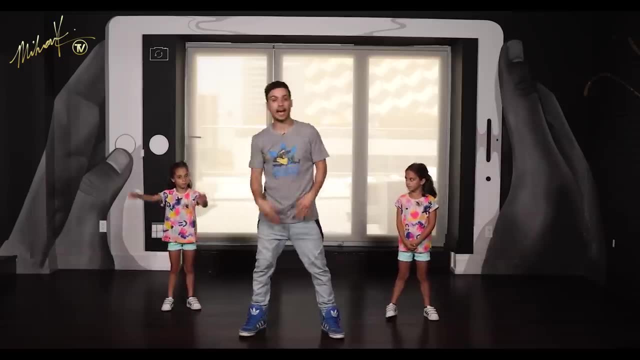 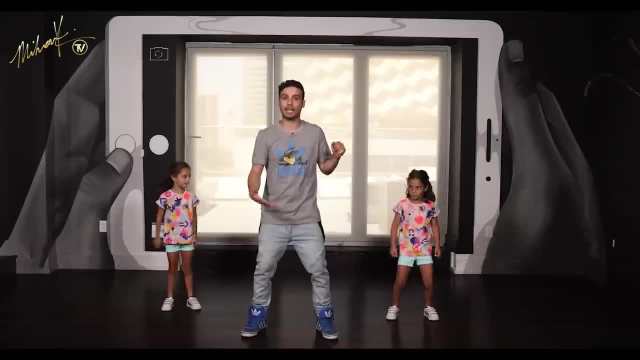 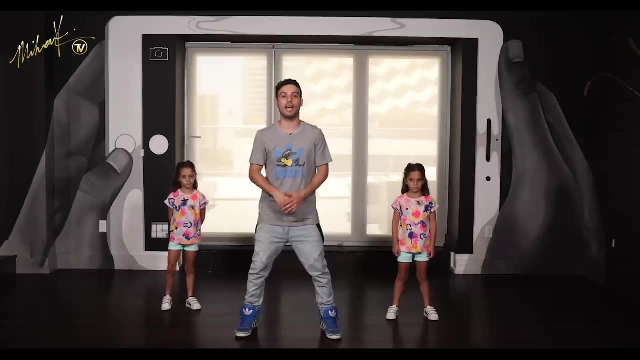 bend your knees. your knees are going to go down, down, down. that's your bounce. you're going to use the arms and move side to side. let's do it once, girls. let's show them five, six, seven, eight. 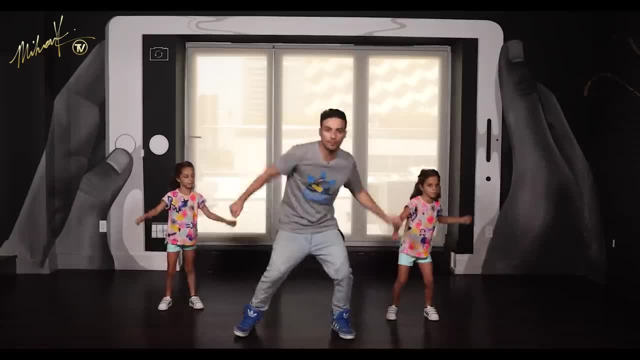 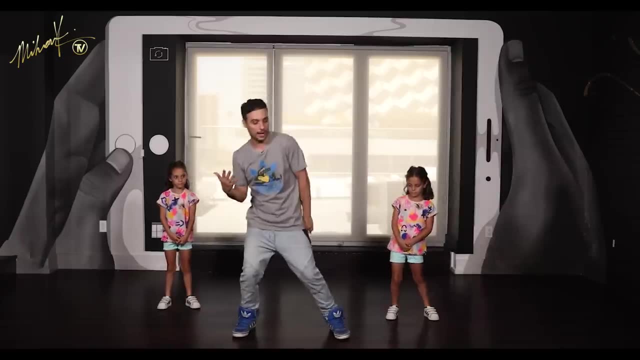 we're going bounce two, bounce four, bounce six and bounce eight. perfect, so make sure we're bouncing all the time. yeah, bounce to the right, bounce to the left. use both knees and arms. 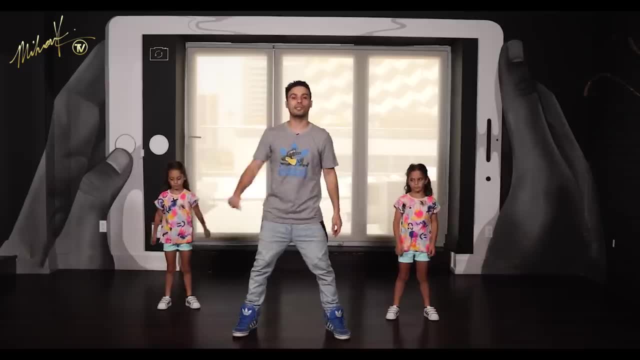 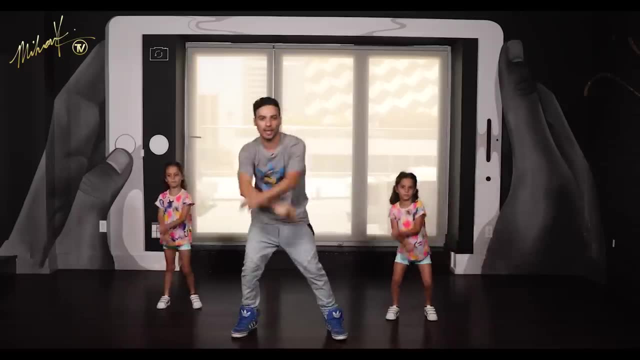 continue to do the same thing. let's do it again, girls. five, six, seven, eight. go one, two, three, four, five, six, seven, eight. good, here we go, let's do it again. five, six, seven, eight. 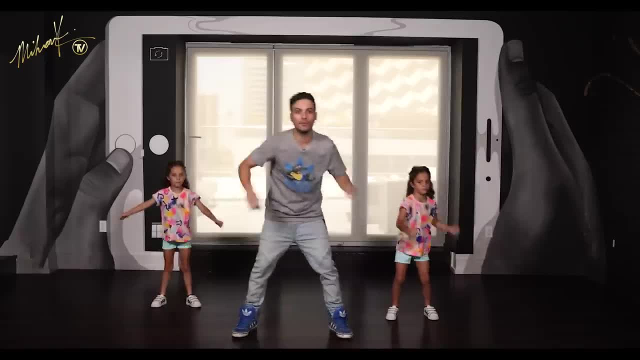 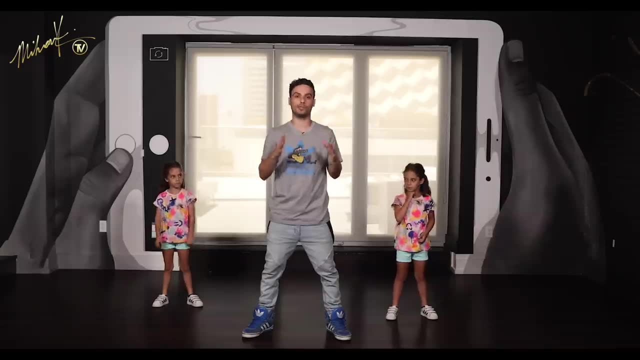 go one, two, three, four, five, six, seven, eight. good, so we're done with step number one and we're done with step number two. let's put these two steps together before we move on. okay, from the very top. 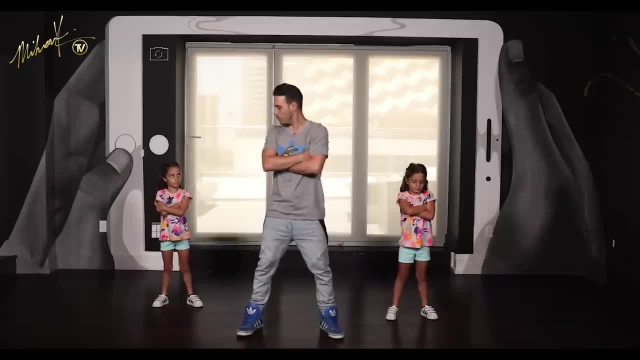 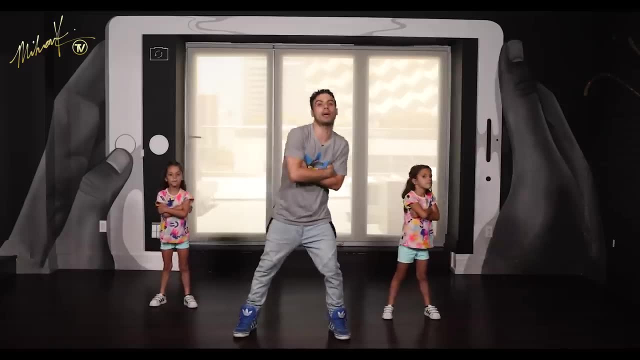 make sure feet are apart, arms crossed, here we go. you ready, Lily, you ready Sophia. here we go side to side. six, seven, eight go, bounce, bounce, bounce. and bounce, bounce, bounce. 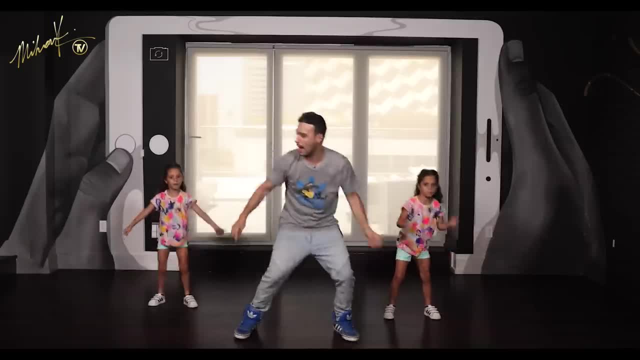 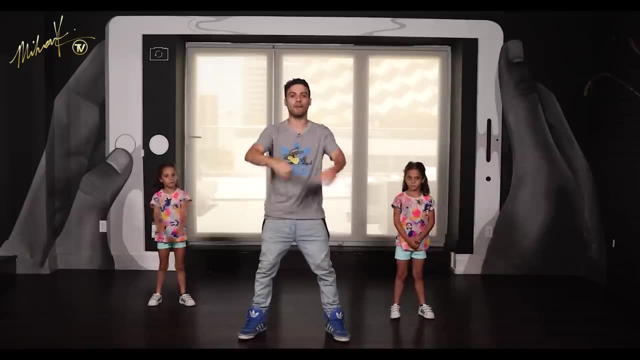 and one, two and three, four and five, six, seven, eight. good, one more time and we'll move on to step number three. okay, here we go. five, arms crossed, six, seven, eight, go, bounce, bounce. 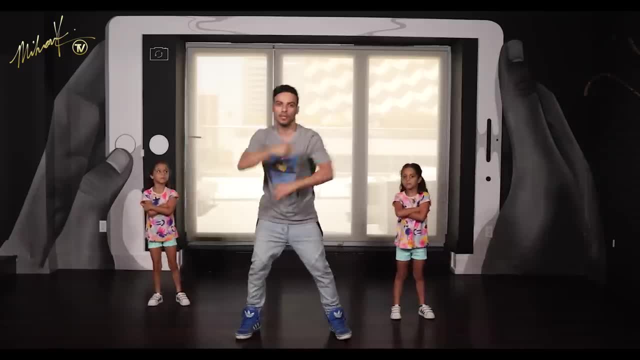 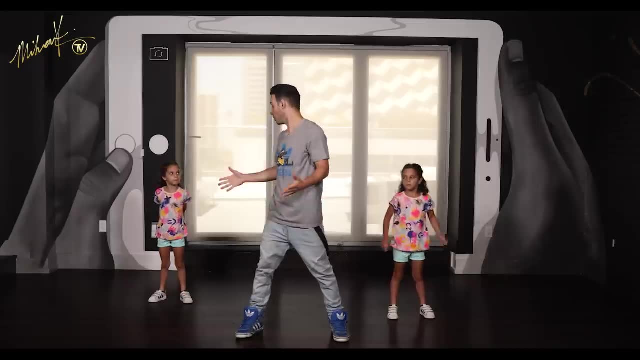 double and bounce, bounce, double and one, two and three, four and five, six, seven, eight. good, from here we're going to move on to step number three. step number three. it gets a little tricky. 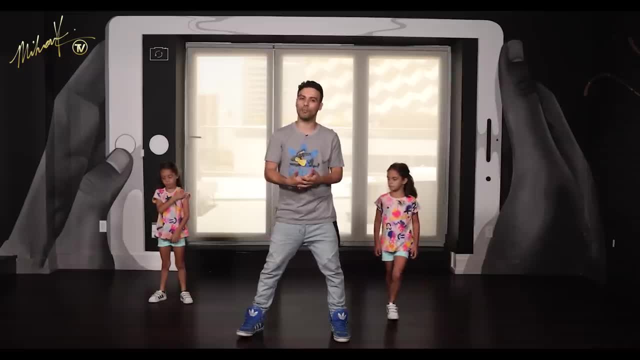 we have to make sure we're using our body, but if you still have a hard time with it, that's fine. just make sure you're doing the arms and the head okay. so we're stepping to the right side. we're. 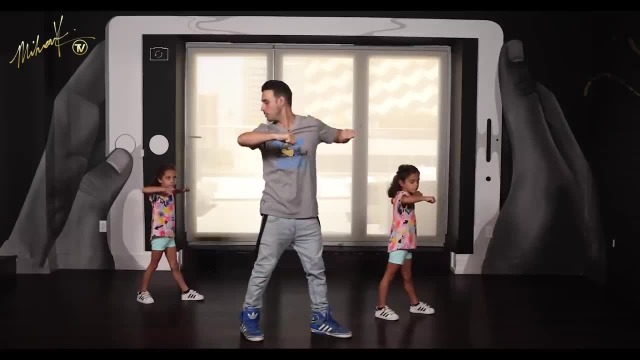 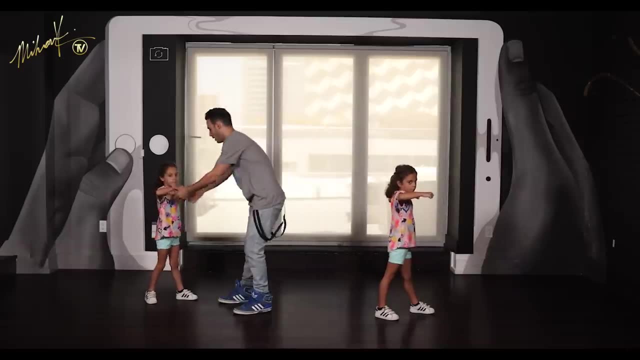 going to pull the arms back. one right arms right here. you got it, Lily, good job. now make sure the arms don't come in and you have it fully out, just like Sophia. perfect and Lily right here. 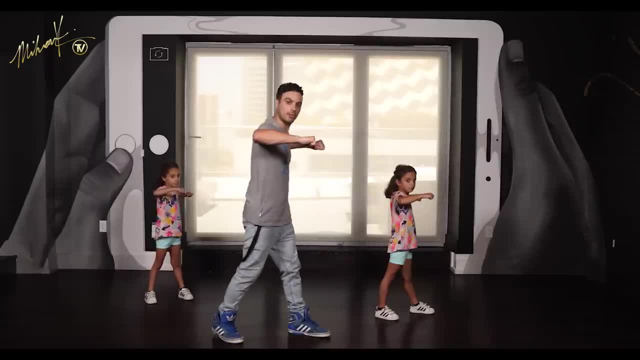 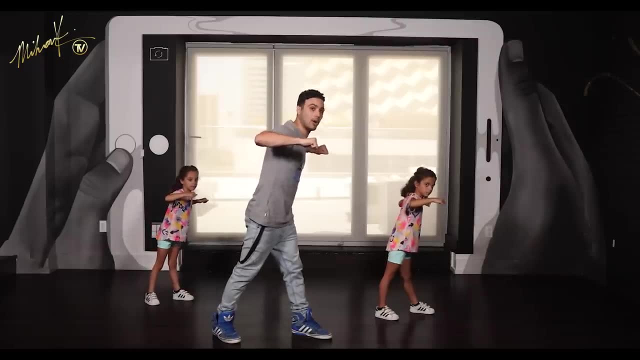 arms strong. good, here we go. we're looking straight. arms are right here. so this is one. now you're pulling back the arms, but you're leaning forward a little bit, and then, when you extend the arms, you're going to lean back and then you're going to come forward and then your 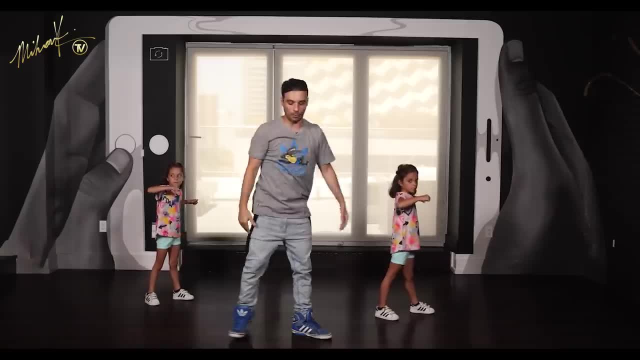 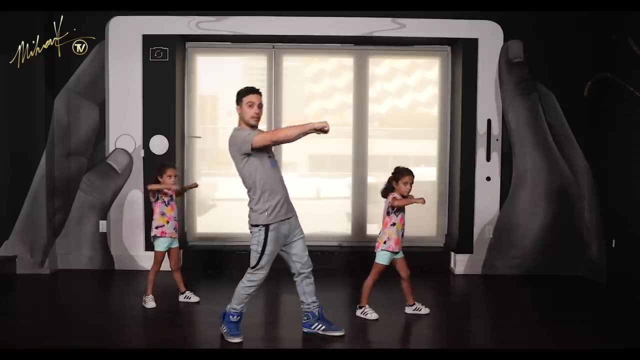 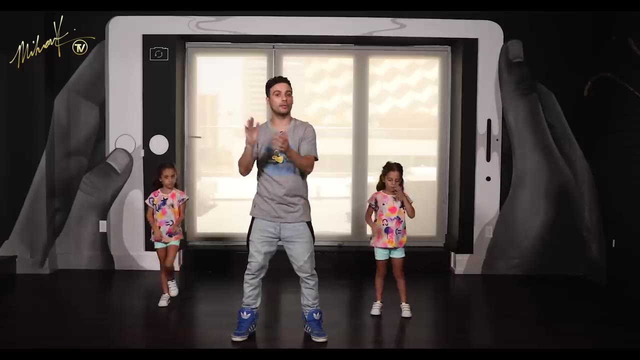 head is going to go up down. okay, let's do that one more time. we just finished the cross. six, seven, eight. we're stepping one, two and up down. okay, let's do that one more time. your rhythm is one, two and three, four. 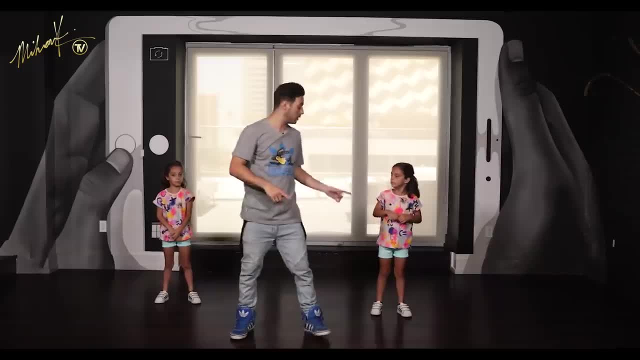 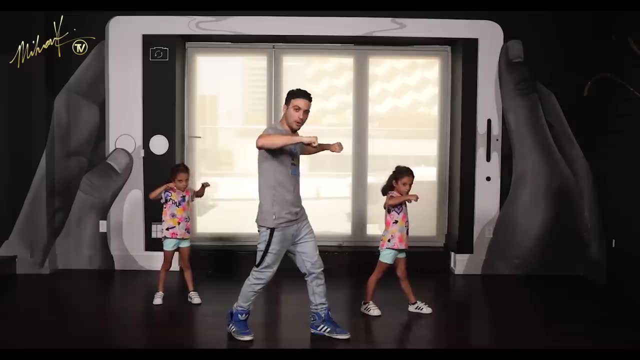 one, two and three, four. okay, let's do it with that rhythm, girls. here we go: five, six, seven, eight. we're going one, two and three, four. good, let's do that again. five, six, seven, eight go: one, two and three, four. good, also when you're. 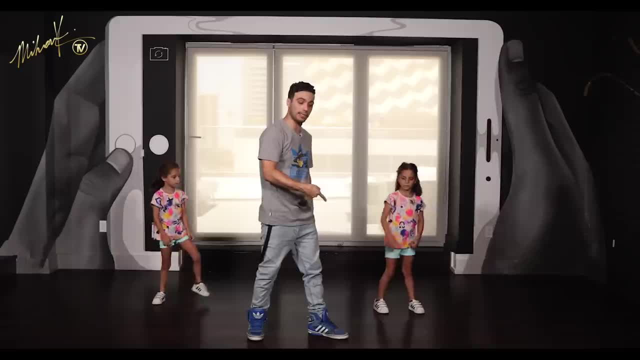 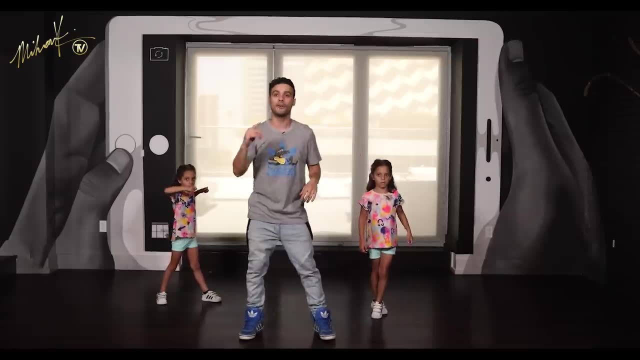 stepping to the right side. make sure you pick up your right leg. boom, you step in place, pull the arms back. right, girls, let's do it together. step in place, pull the arms back and then keep going. five, six, seven, eight, go one, two and three, four. 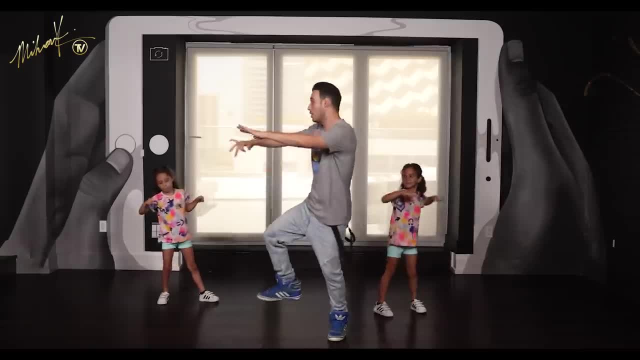 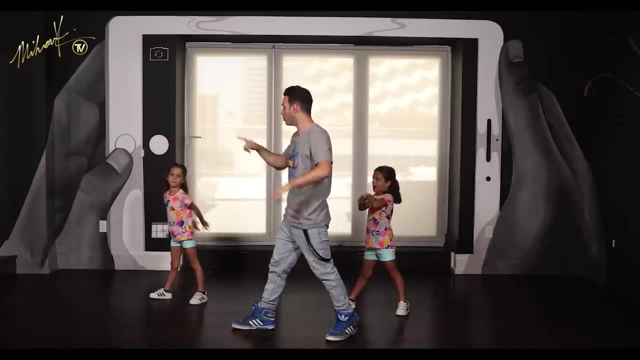 now let's do the same thing. moving to the left side, here we go. five stepping with the left leg. move back front up down. good job, let's do a couple of times. on the left side: girls, here we go. 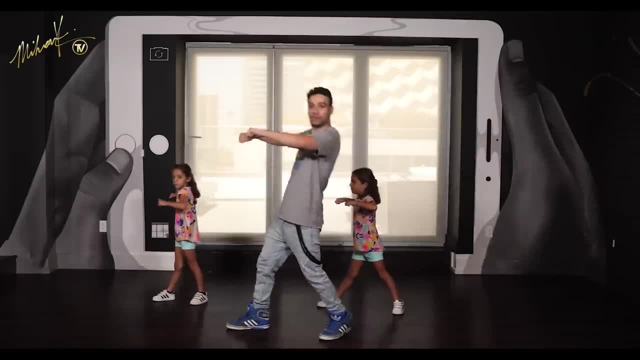 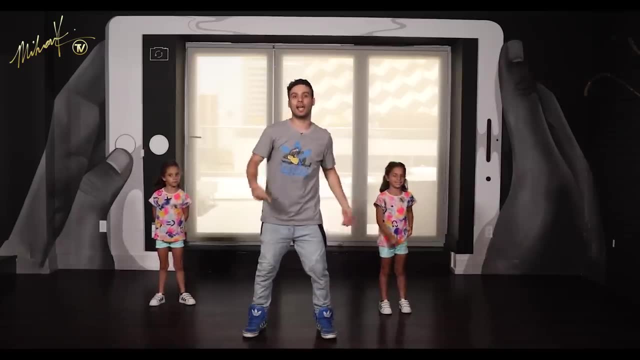 six, seven, eight, go one, two and three, four. good, let's do it again. left side: only five, six, seven, eight, go one, two and three, four. perfect, let's connect the right side. 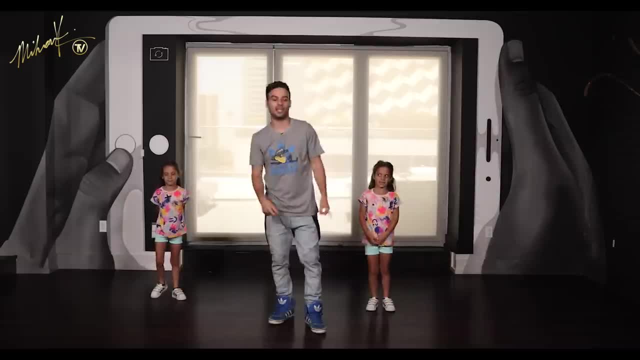 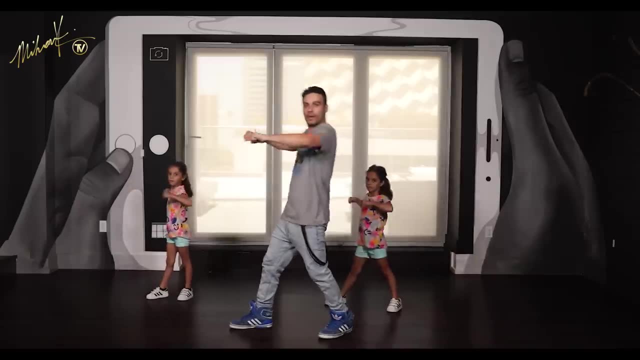 and the left side together. okay, here we go. five, six, seven, eight, go one, two and three, four. one, two and three, four. good, so remember if you're doing it with your daughter. 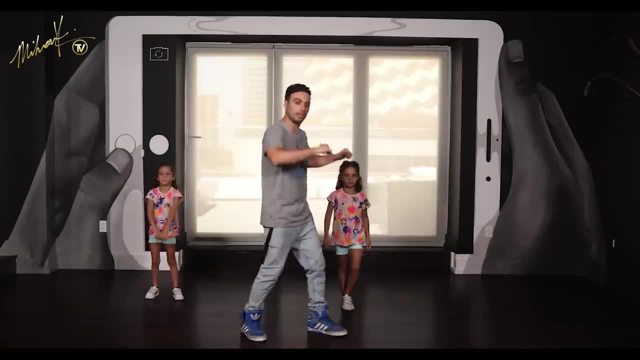 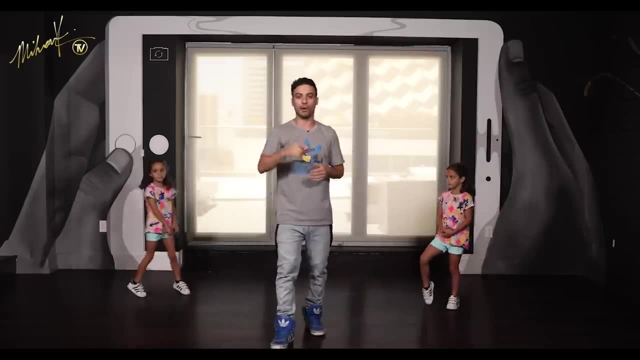 your nephew, your cousin, anybody really young, and they're having a problem with the body movement. let them just do the arms and the head and then, little by little, they'll open up and also be able to lean. okay, so let's go back, let's do step number one, step number. 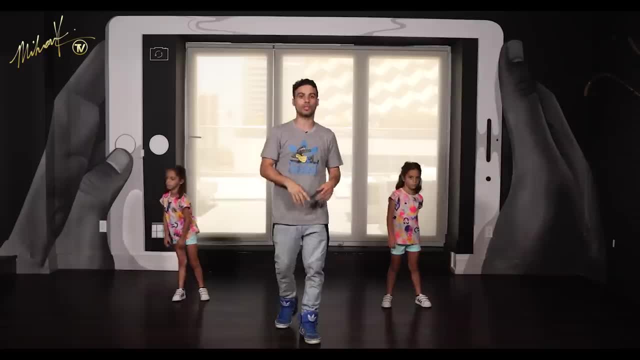 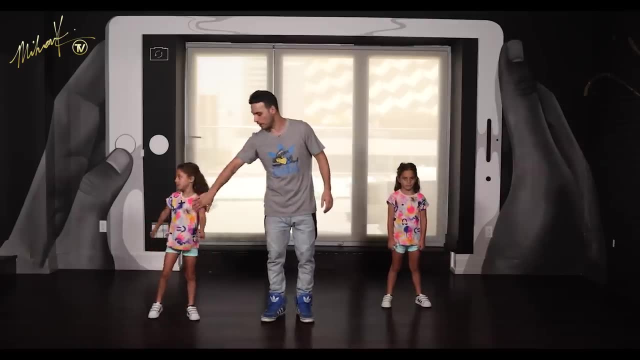 two and step number three together, and then we got one more count. this last part is fun and easy and we're pretty much done with the routine. okay, Here we go. let's go from the very top. you ready, you ready, I'm gonna, we're gonna assume. 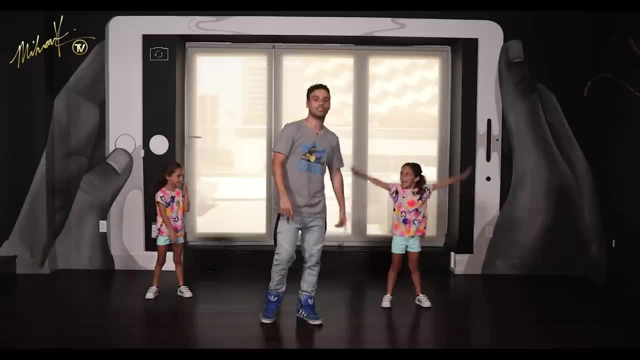 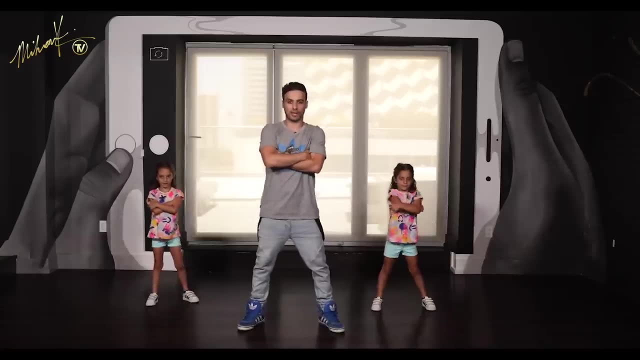 the swinging means: yes, are you ready? yes, she's gonna swing as well. here we go five, six, from the top feet apart. here we go, arms crossed. hopefully you guys are ready too. here we go, six, seven, eight go: one, two, three, four. and one, two, three, four. 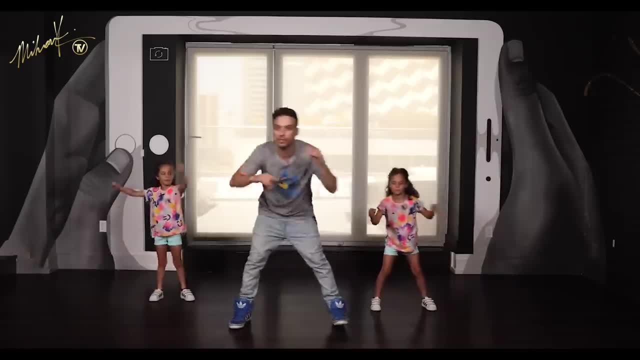 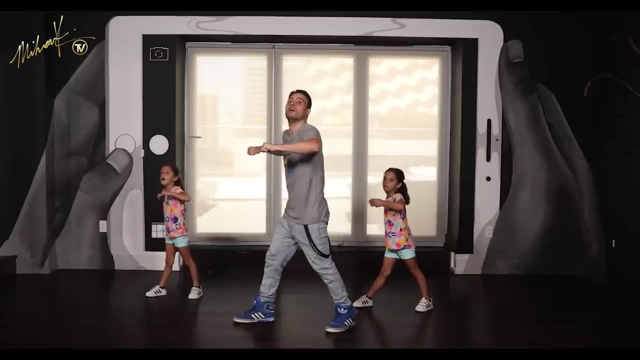 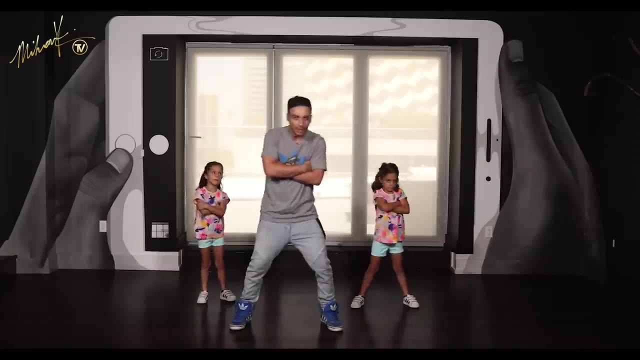 and bounce and bounce and bounce And step, step, step up down, step, step, step up down. perfect one more time, just like that. five, six from the top go: one, two, three and four. one, two, three and. 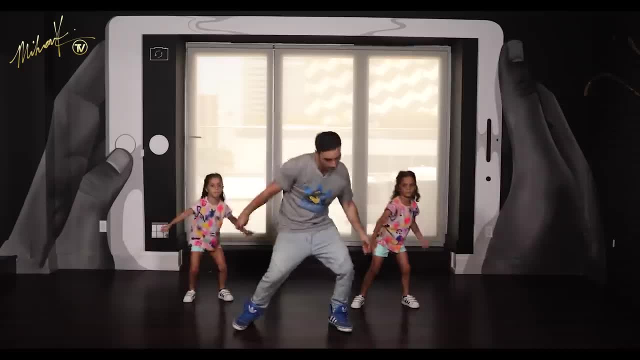 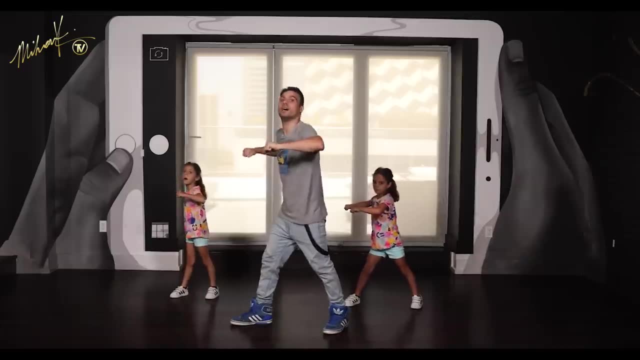 four: go, bounce and bounce and bounce and bounce. good, hit, hit, hit up down. hit, hit, hit up down. good, This last part: stay in your place, arms up, here we go. you're gonna walk around yourself. 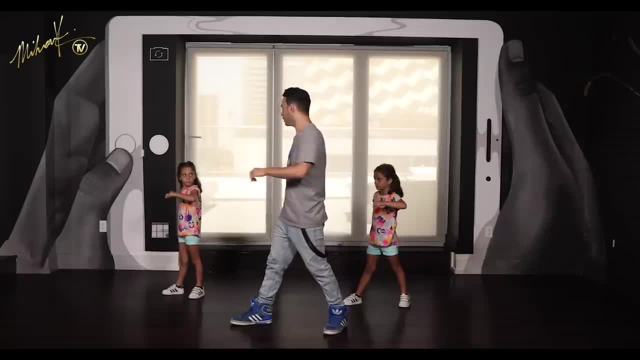 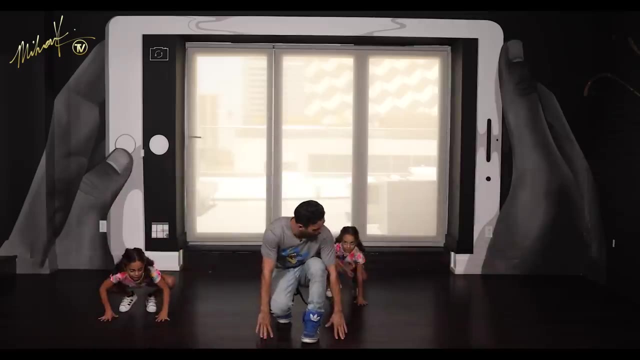 for four counts. in this case, we're gonna have Lily travel this way, Sophia's gonna go take her place. okay, four counts, and then we're all gonna drop on count five. here we go, let's show them: girls seven, eight, walk one, two, three, four down five, good. 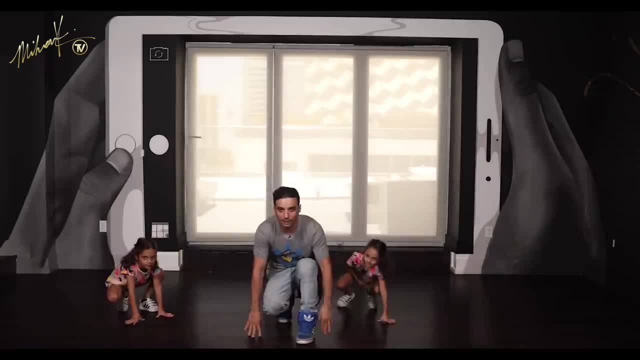 come a little to the side. there you go five. so when you go down you can do whatever you want. it's free. You can come down here with two hands on the floor. you can lean to the side, you can do. 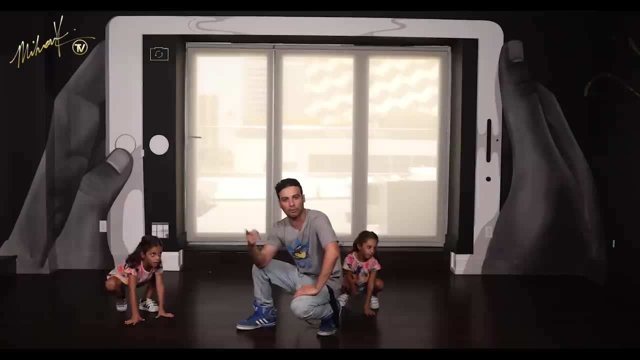 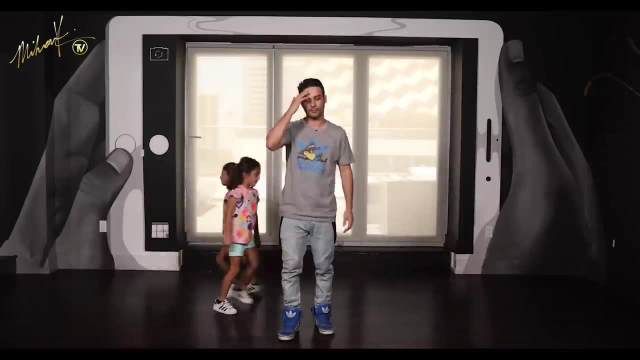 whatever you want, it's free, so don't think too much about it. just move around your friends or around your partner and then just come down. let's do it again. girls switch back, here we go, so just the walk around part. okay, we just finished here and we went up. 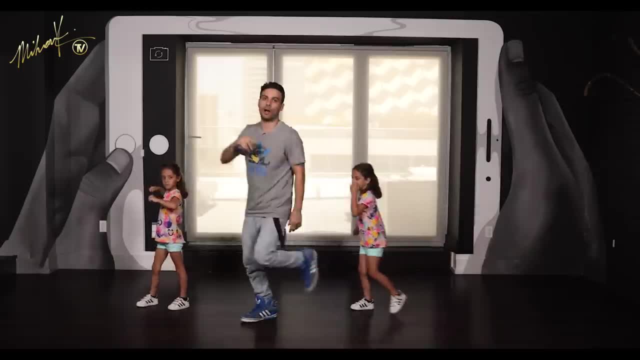 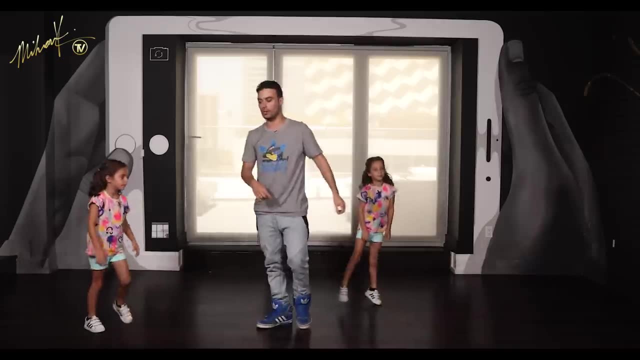 down. now we're gonna walk around six, seven, eight, walk one, two, three, four down. good, Now let's do that again. switch girls one last time and then we're gonna show them. 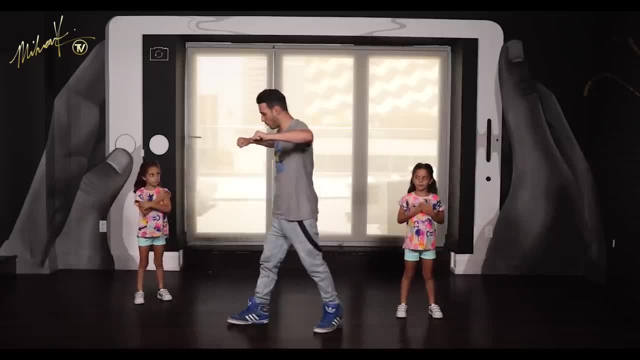 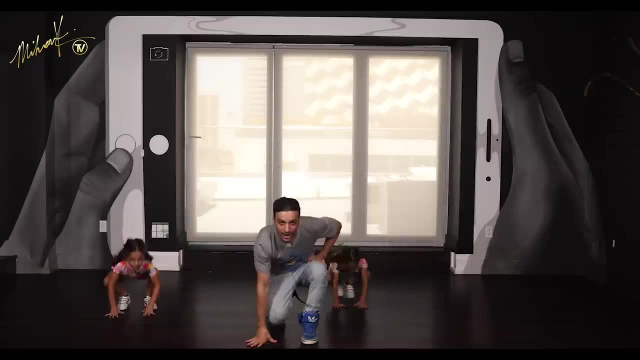 the last part. okay, here we go, five, six. let's go from here: five, six, seven, eight. walk around: two, three, four, down five. we're gonna hold six. okay, so five and six. 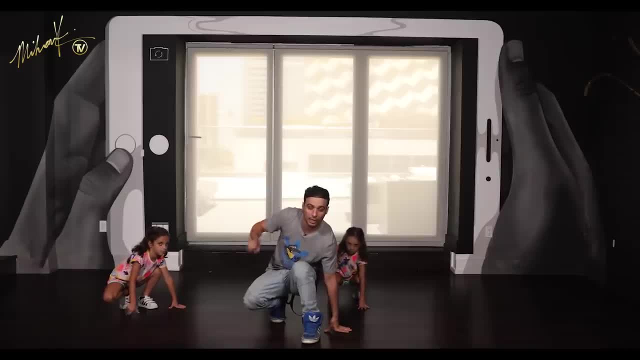 no movement. we're gonna hold five, we're gonna hold six, you're gonna travel back up on seven and eight and it's free. you can do whatever you want. I'm kinda gonna wave my arms coming up. I don't know what Sofia's gonna do. it'll be a surprise. what are you gonna do, Lily? 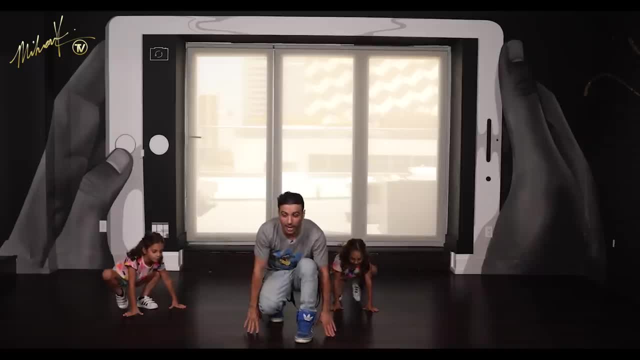 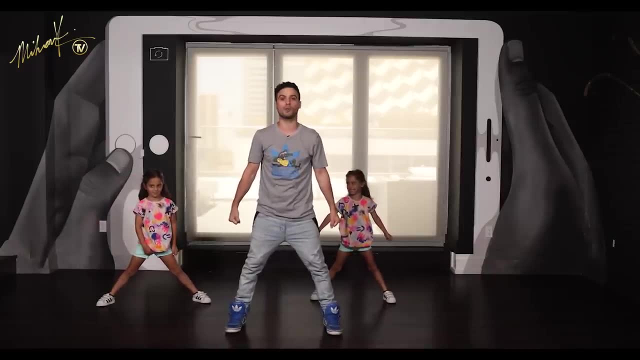 She doesn't know yet. Here we go, let's give it a try. we're holding five, six, come up seven, eight, jump one and that's it right there. that's gonna be our last pose and we're gonna finish it there. 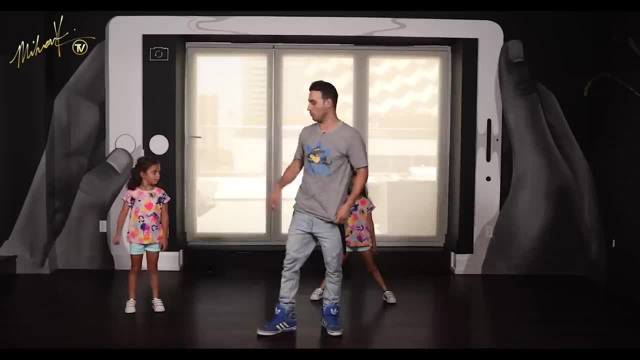 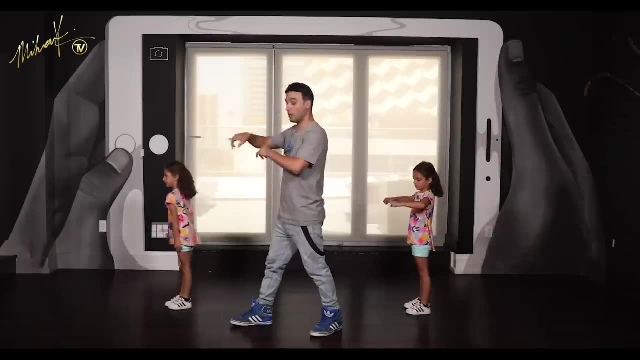 that's your four eight count routine. okay, really simple: all grooves. let's do that last part one more time. girls, let's go from here. switch places one more time. when we walk around, we go down. we're gonna hold. 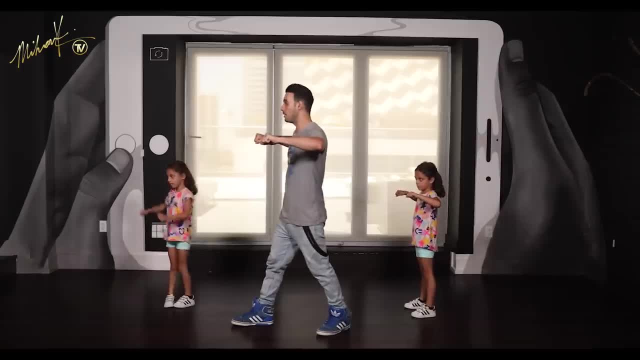 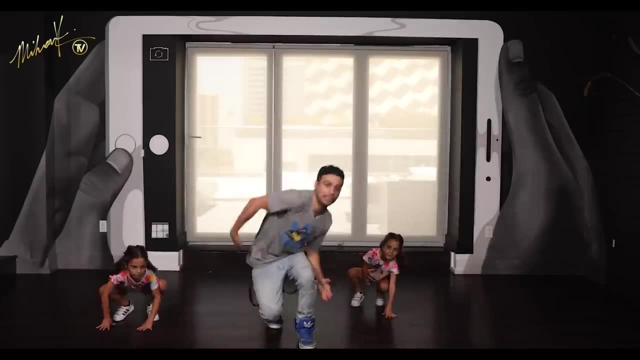 Jump, Jump, Jump, Jump back up and then hold on one together. here we go. five, six, seven, eight, walk around two, three, four down. five, six come seven, eight, one. all right, guys, let's. 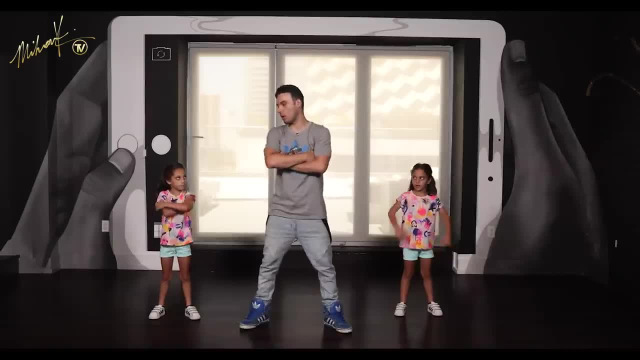 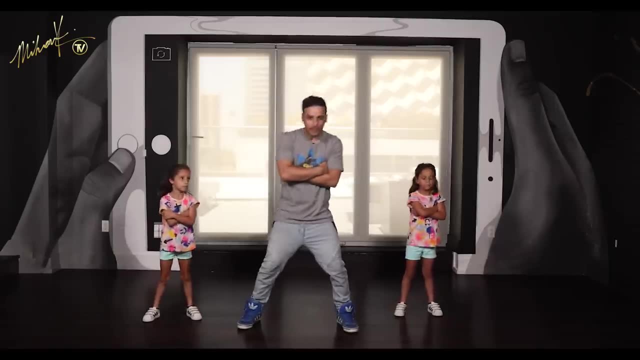 do it again from the very top. here we go, feet apart, arms crossed, five, six, seven, eight. go one, two, three and four go. five, six, seven, eight, go bounce, make it big. 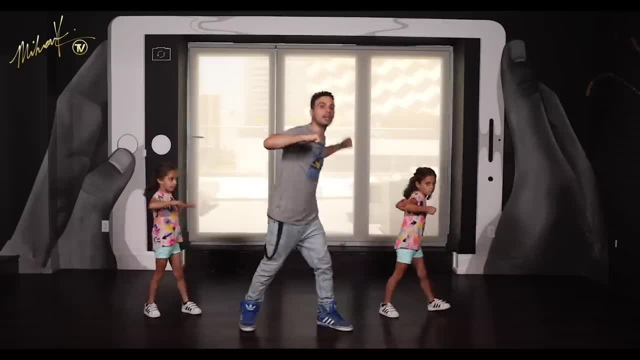 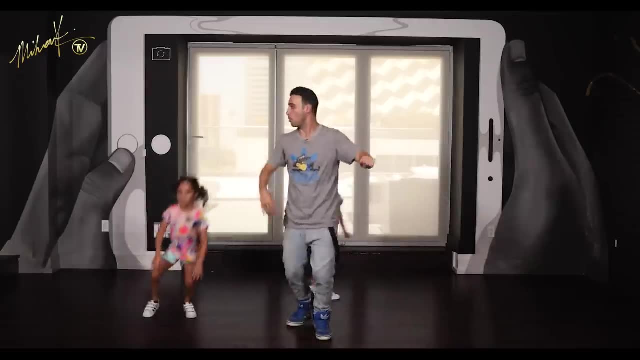 and five, six, seven, eight Go. one hit hit up down, one hit hit up down. walk around two, three, four down. five, six up seven, eight hold. 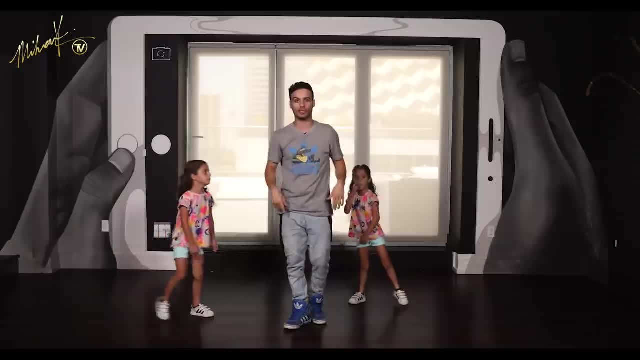 Nice, Let's do it one more time, just like that, guys, and then we'll try it with music together. Here we go, girls, switch back. this will be the last time, and then we're gonna do it with music. 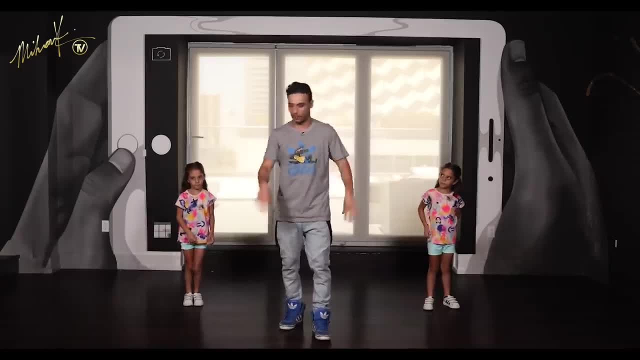 Let's make this one really strong, bring out all that energy. here we go, five feet apart, arms crossed, six, five, six, seven, eight go one hit hit up down. one hit hit up down, walk around. two, three, four down. five, six up, seven, eight hold. Nice, Let's do it one more time. just like that, guys. and then we'll try it one more time. just like that, guys, and then we'll try it one more time. just like that, guys, and then we'll try it one more time. Here we go, boys, we're gonna do it with music right now. traffic and one eight. get into order slowly, few. Alright, let me just pass my Three, two, two, one. go girl, touch the ground, and then we're gonna come up, and then. Now don't could on it's own, got it. Now don't could on it's own, got it. Yeah, and we're gonna hit it little high over three, two, two and comes in pushing unalterable alleys. 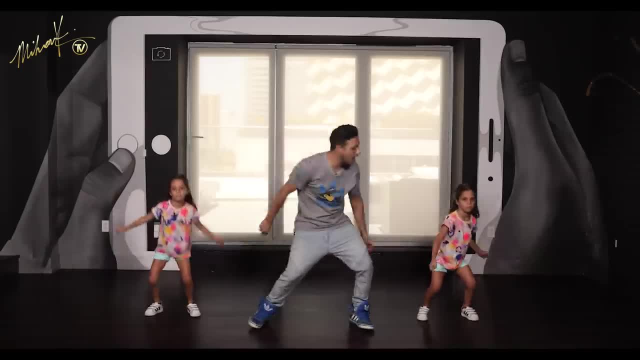 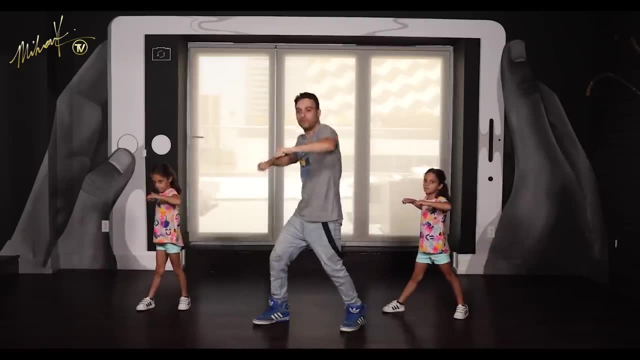 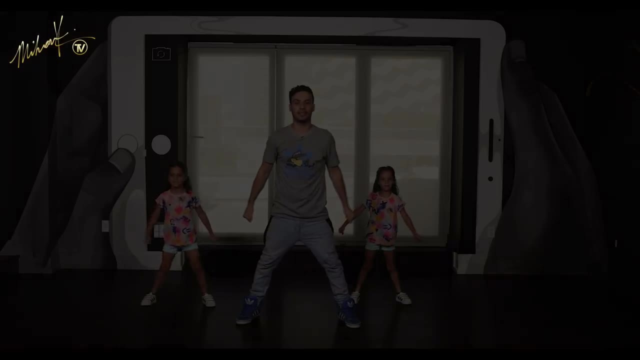 Alright, so let's work it again. rotate the dirt, Yeah, so let me shake hisちょco toe two and hit four and five, six, seven, eight. go one, two and three, four, one, two and three, four. walk around two, three, four, down five, six, seven, eight, hit. all right, guys, here we go, let's do it. 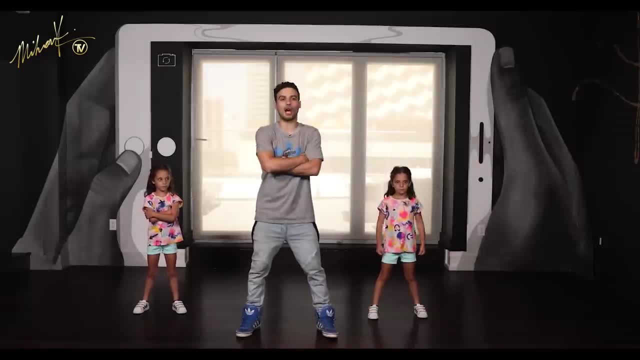 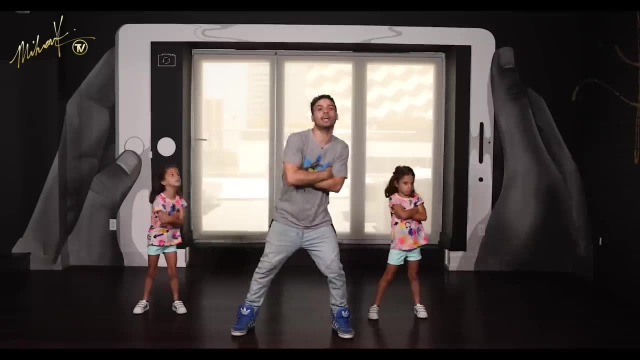 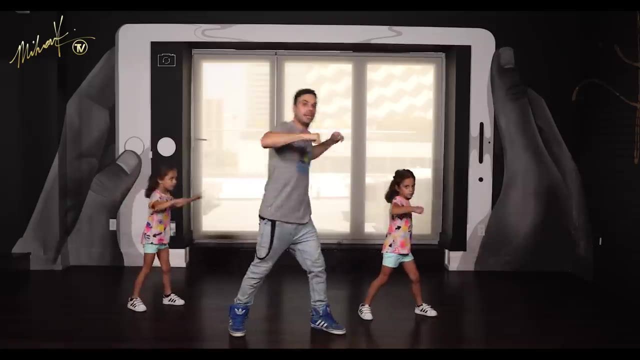 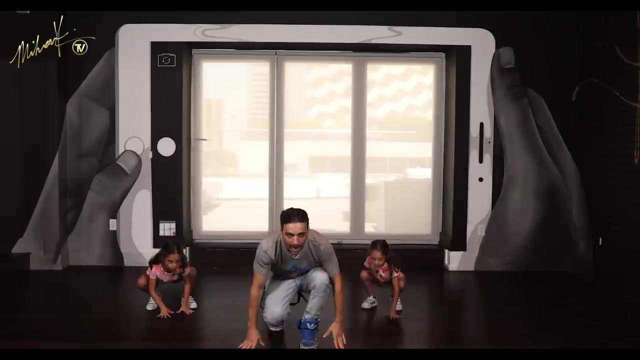 with music. we're ready. feet apart, arms crossed, and five, six, seven, eight go. one, two, three, four, make it big. six, seven, eight, go bounce. two, three, four, five, six, seven, eight, go, hit, hit, hit up down. hit, hit, hit up down. walk around, two, three, four down, wave and jump. 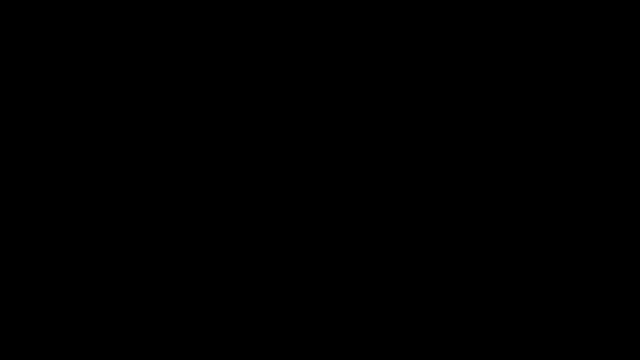 one, two, three, four, five, six, seven, eight go. one, two, three, four, five, six, seven, eight go.